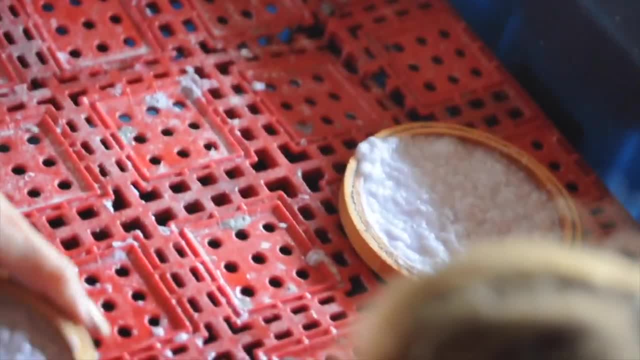 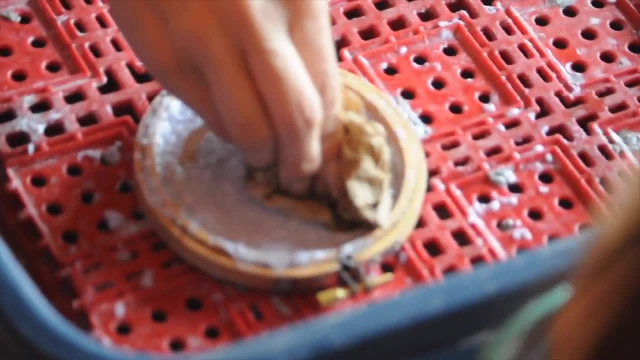 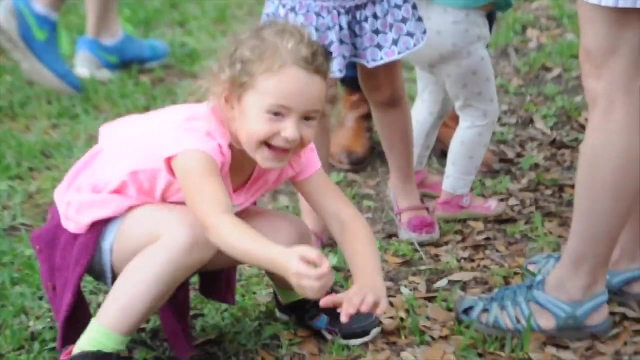 And here we're just kind of trying to force the water to come out. Another way that we can help of doing this is just getting a piece of paper and press Just a little press. Okay, so you want to peel it? Yeah. 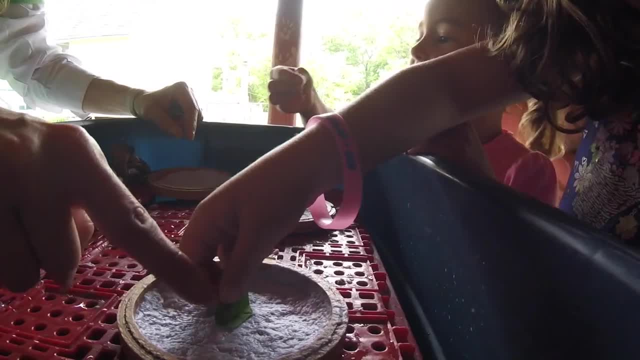 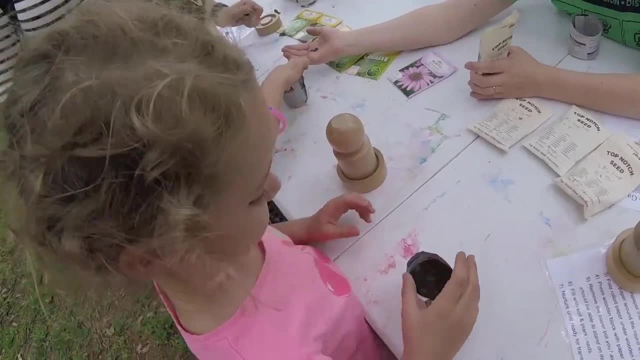 Okay, Want to see bud Here in the middle. Okay, It's like heart eyes. Yeah, Do you like it, Amelia? How big do you think it's going to get? I don't know. You think it might get like this tall. 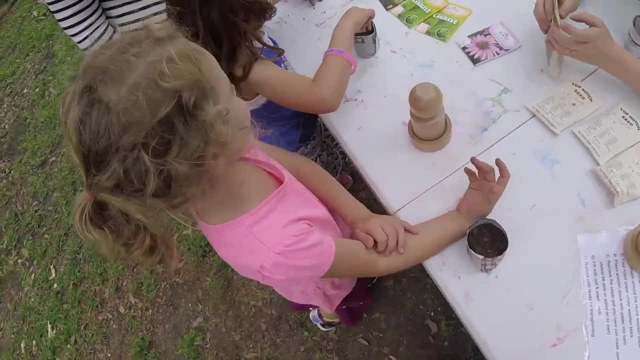 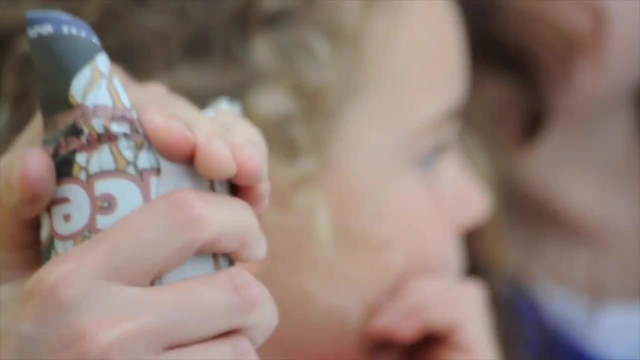 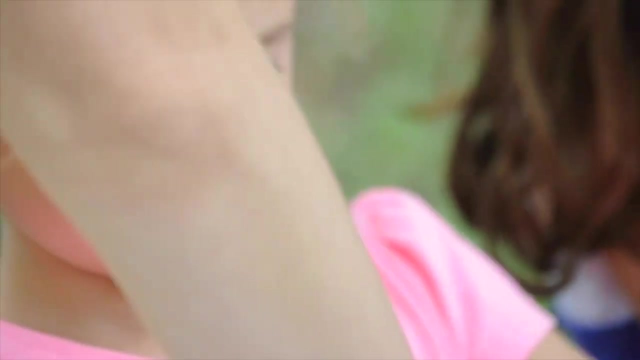 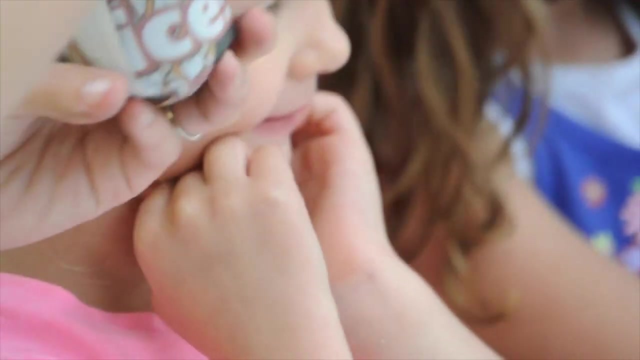 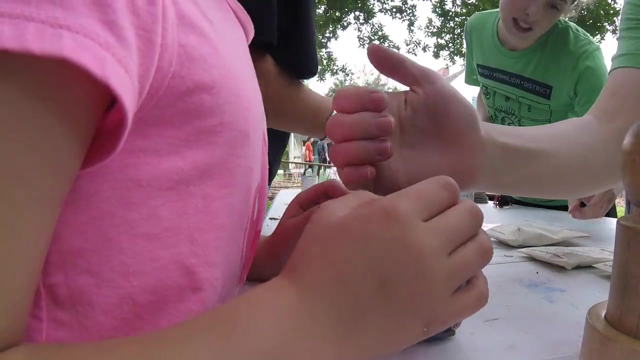 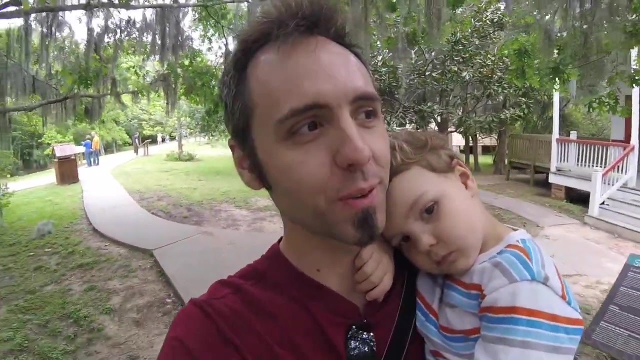 Whoa, That would be a big flower. huh Yeah, Push hard. You made a pot. Go get some dirt. All right, guys Having a fun time. There's so many projects to do. They made little paper pots. 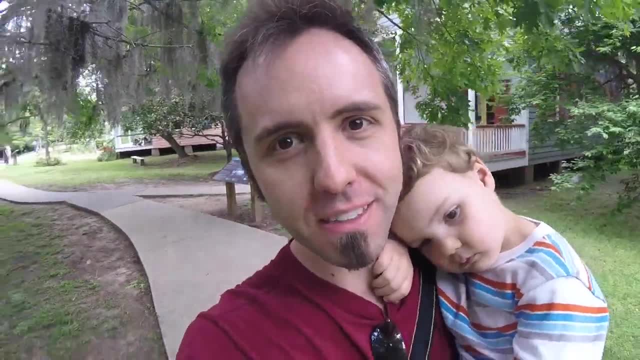 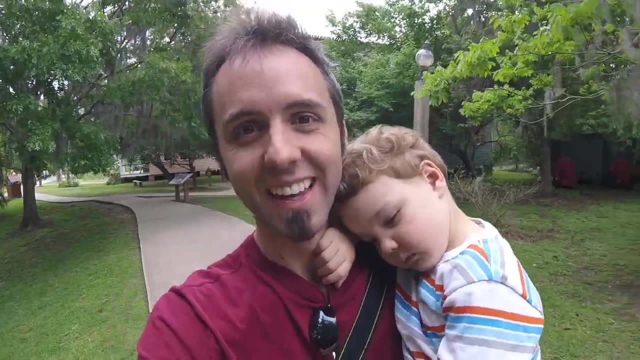 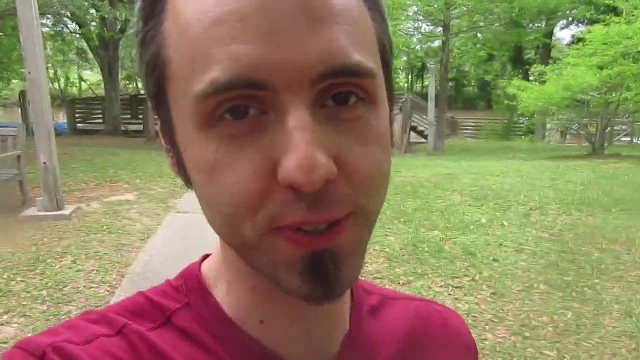 They made recycled paper and leaf rubbings, fish rubbings. You having fun, bud, Yeah, You getting tired? Yeah, So we're going to go eat some lunch now. The university here owns an Airstream and they made a museum out of it. 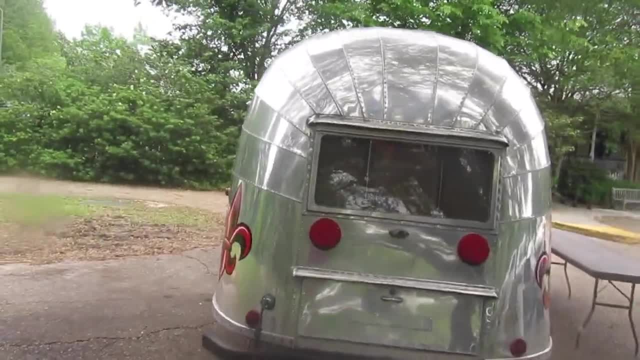 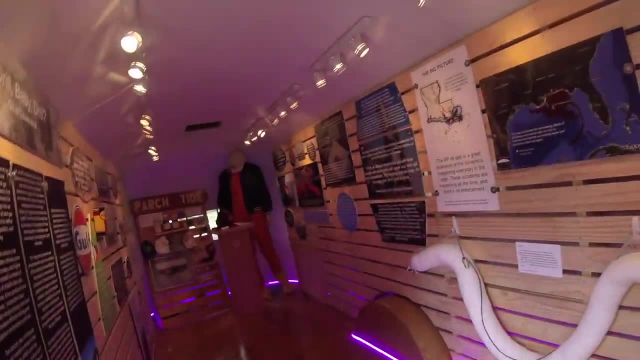 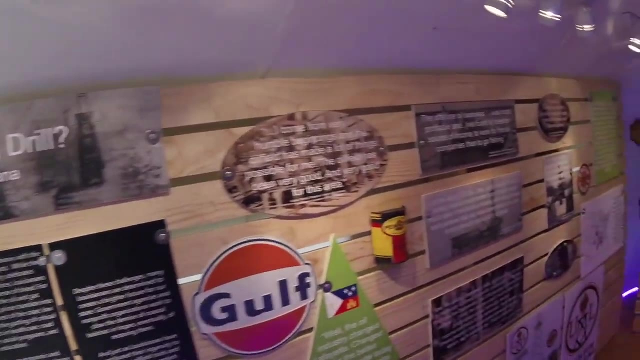 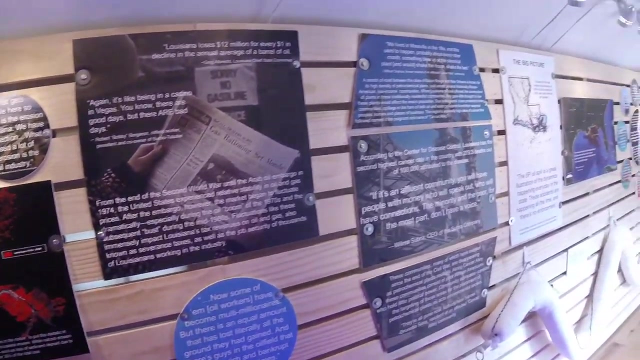 It's an old one. It looks like maybe 70s, I don't know. It's fancy Beautiful. So this is inside the Airstream and I guess it's a Louisiana museum, I'm assuming. I guess it's all based on the oil industry. 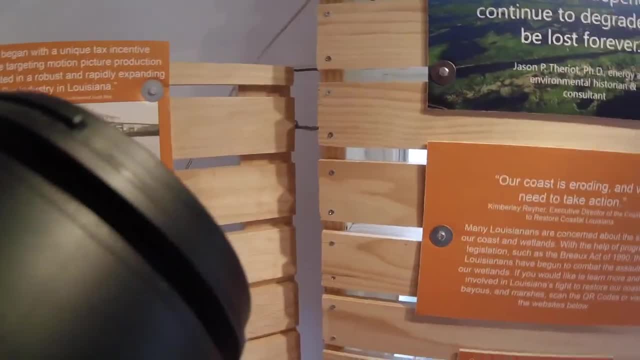 Do you guys have any questions about it? I'd be happy to answer. Is it just about drilling? It's about the oil field. So right here you're going to have sort of like. the theme of it is like: what did the 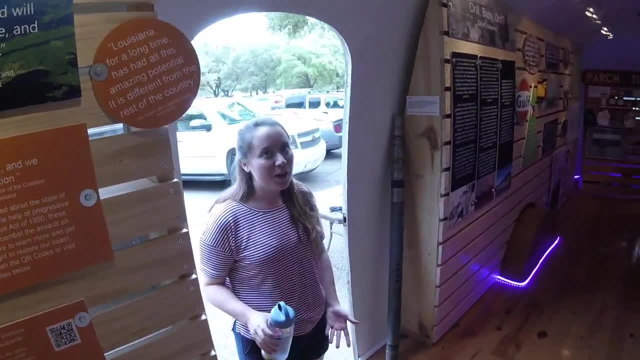 oil field do. I don't know, I don't know, I don't know. It's like: what did the oil field do for Louisiana, What has it taken away from Louisiana And how we feel we can diversify. So I was one of the students who created this. 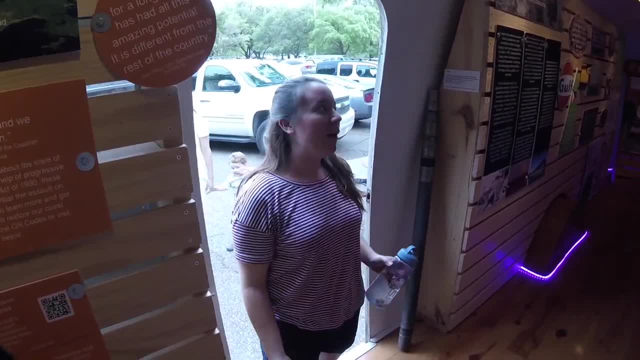 So if you guys have any questions about it, I'll be able to answer it. And I saw you were looking at, kind of like, how this was mounted into the- Well, actually I was seeing if the windows were open, It was hot and y'all shut them out. 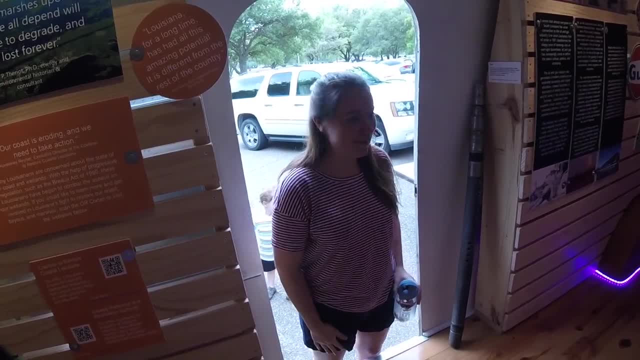 Yeah, That was one of the problems whenever we put these things in here, because we wanted sort of a permanent wall installation for it so that we could hang panels. Do you know the age of the Airstream? I love Airstream. 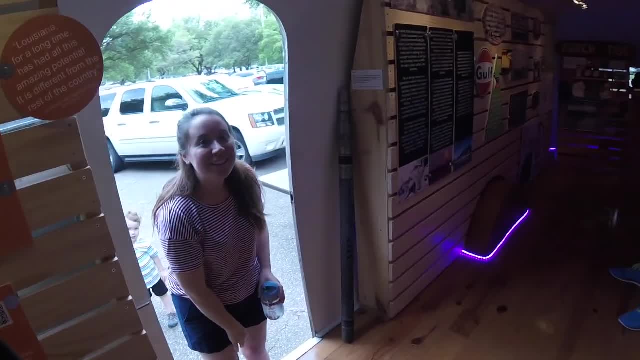 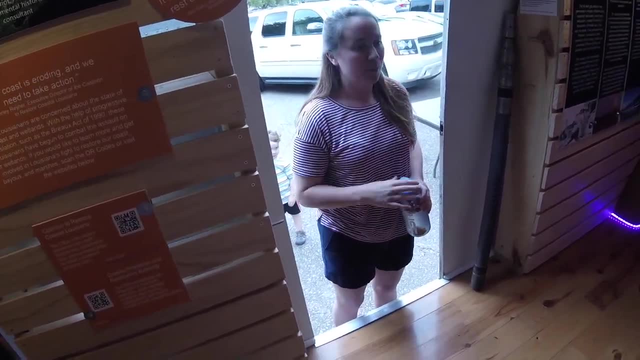 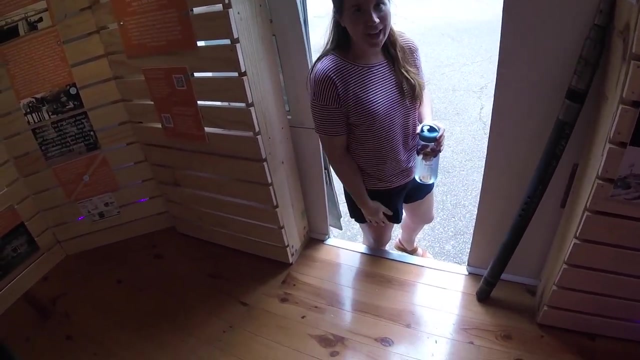 It's 1950s. 1950s, Yeah, So it's a little bit older than the Airstream. It's a little bit older than the Airstream: 1950s, Okay, cool, Yeah, it's 1950s. 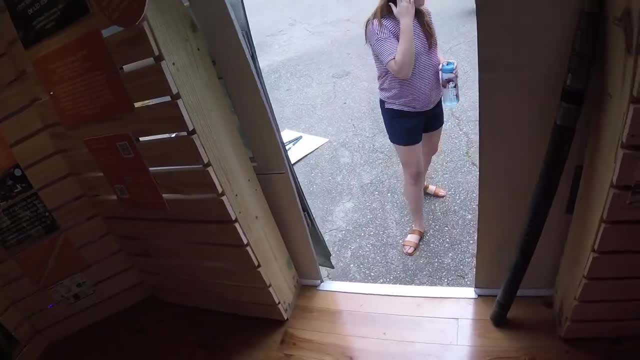 Wow, Older than I thought. We have the panel that just fell down. It'll tell you. It tells you about the Airstream. Yeah, Okay, cool, Awesome, I'll check it out. That's a 1954 26-foot Airstream right there. 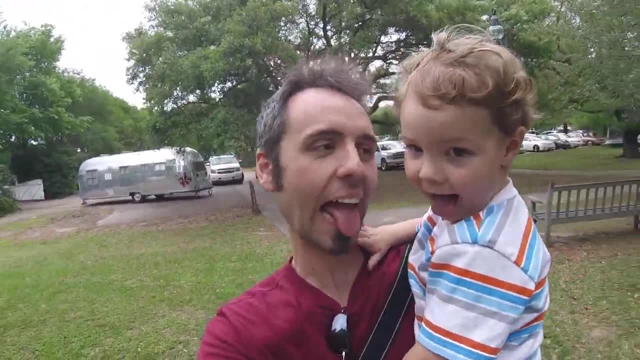 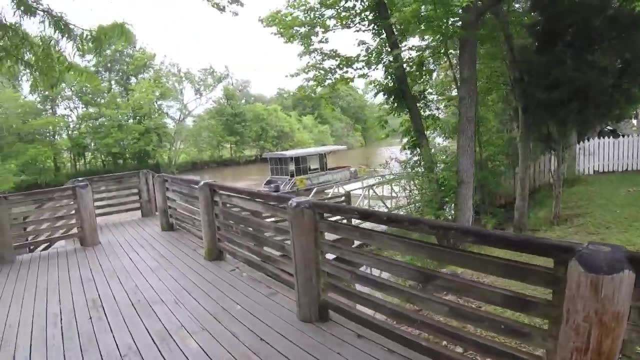 They did a good job, like remodeling it, although it's very hot in there. Did you like the Airstream? Look at that boat. Whoa, It's the calibrated alligator. It tickles, It, tickles, It tickles. 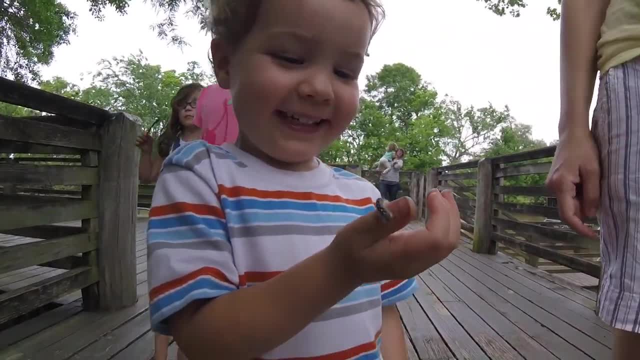 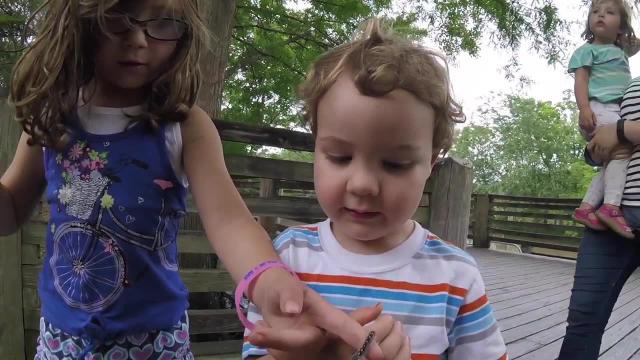 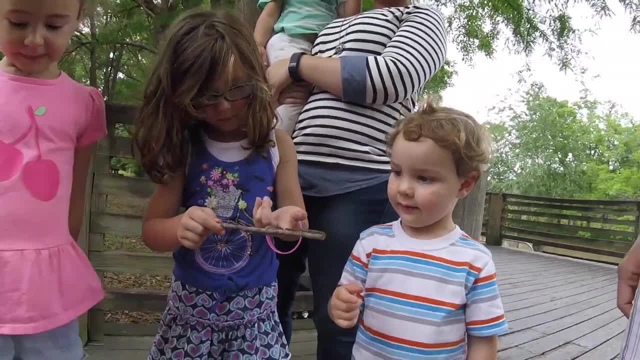 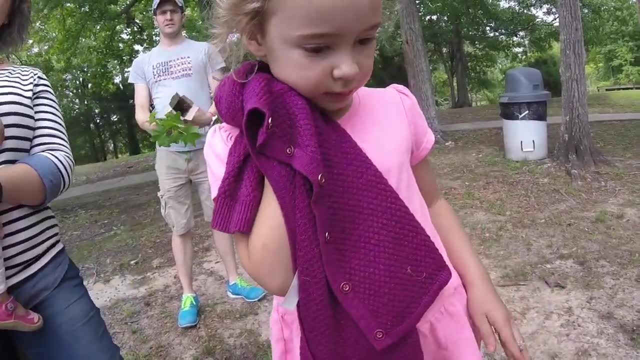 Oh, Kind of got a collection going here. Oh gosh, Great. I think I agreed on two, All right. Well, thank you guys for inviting us. We had a really good time. Yeah, Did you have fun? That was fun. 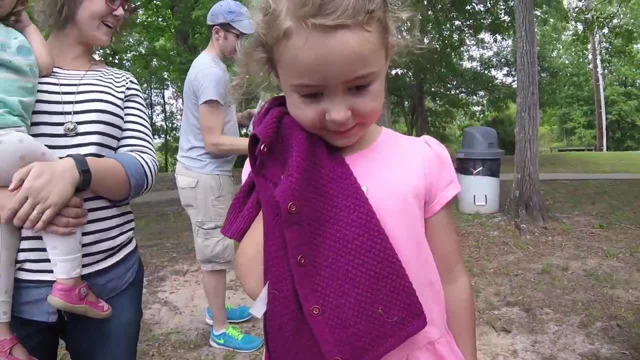 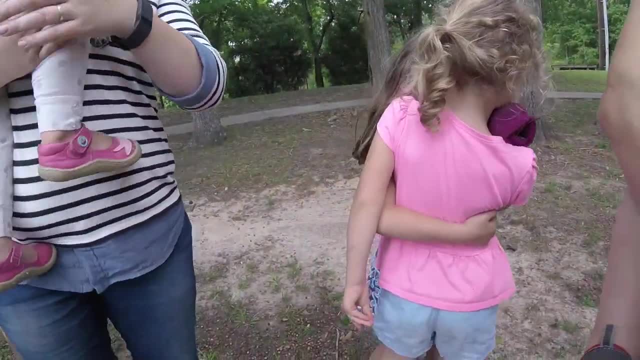 It was awesome. I had a lot of fun. Yeah, Yeah, Yeah, You had fun. Oh, A big hug. Oh, sweet Bye, Violet. Yeah, at festival, I'm sure we will. Yeah, Is that what I heard? 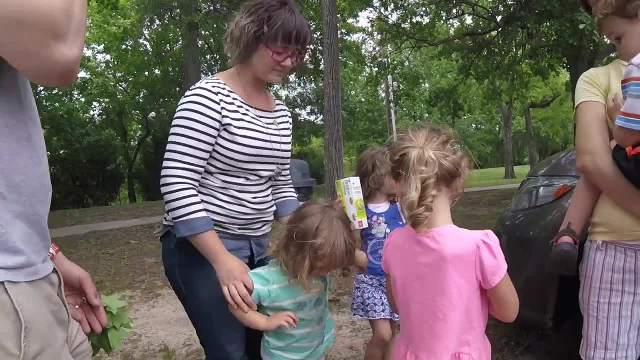 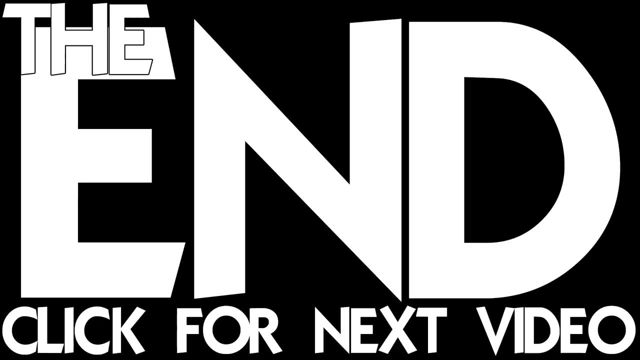 Later, man, He might fall asleep in the car. He wants another hug? Yeah, He will. I think Violet wants another one. He crashes pretty easily. Bye, y'all. It's festival, international time. You excited? Yeah, You like dancing with me? 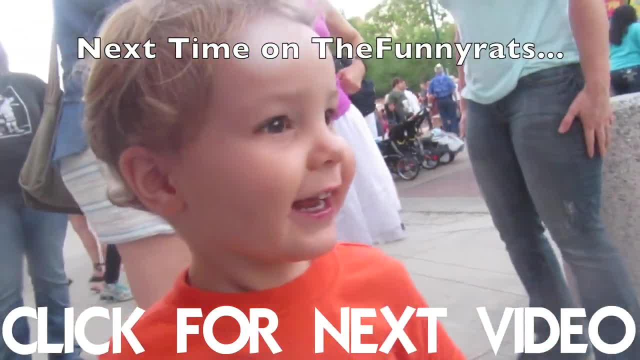 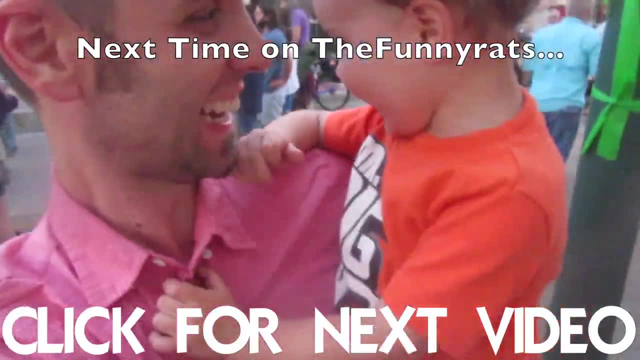 Yeah, Yeah, Yeah, Yeah, Yeah, Yeah. You like dancing with me? Yeah, Yeah, Ha, ha, Ha, ha, ha, ha ha. 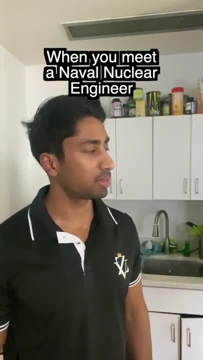 Yeah, I'm just still in the army, man, Just it's going. I'm just trying to enjoy my leave right now, you know, Oh, you're friends in the Navy, Yeah, so it's going to then set me up for.